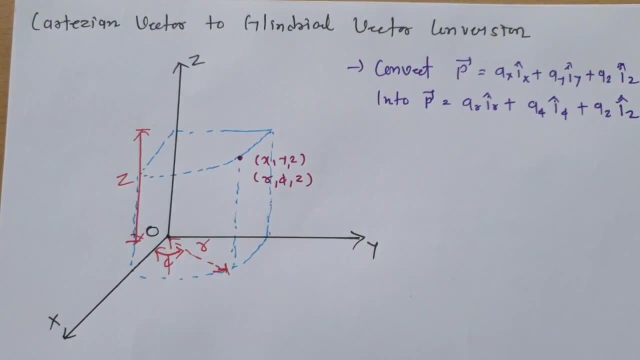 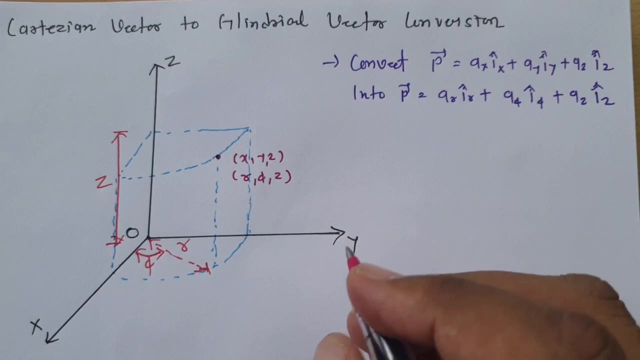 So how to represent direction of R, PHI and Z. So once you know the direction of R, PHI, Z, I think it will be easier to understand conversion. So, direction of R that is there in the radius direction, direction of R that is there in: 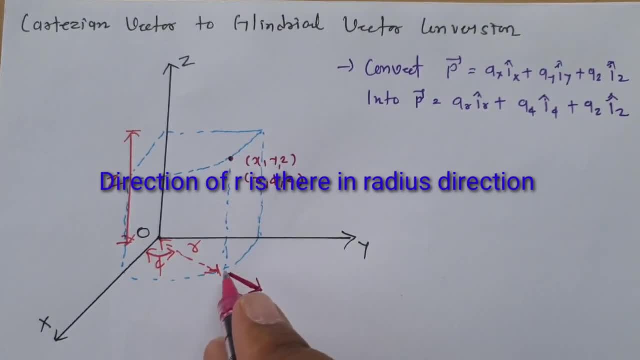 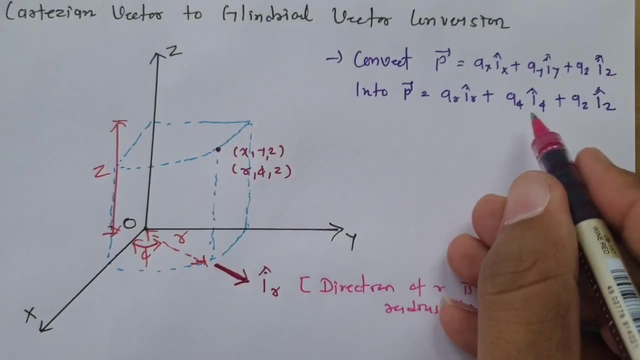 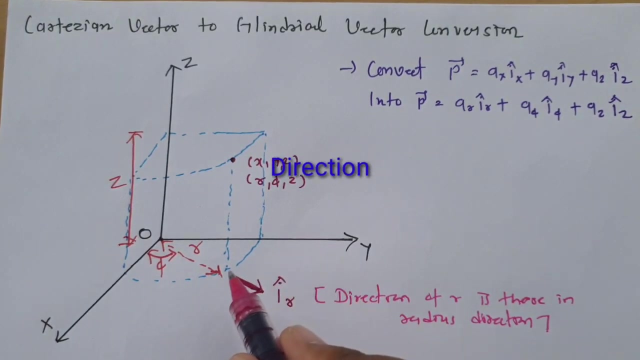 the radius direction. you can see, this is the radius direction at this point, right, so we can say direction of R, that is there in the radius direction. let me mention it IR. Now direction of PHI, that is I, PHI, that is there from X to Y direction and tangent to 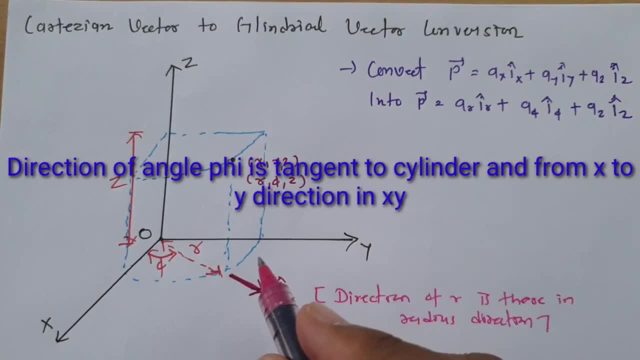 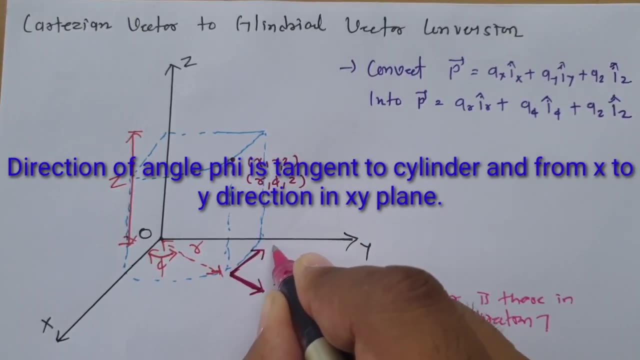 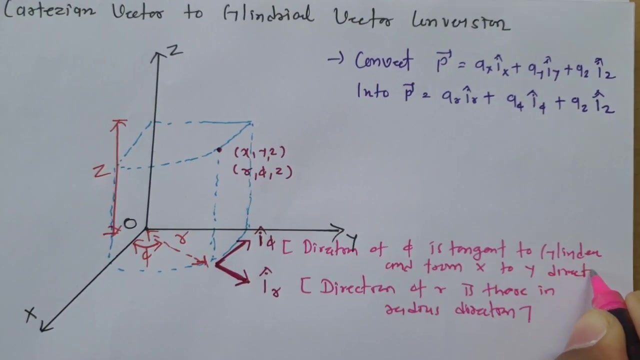 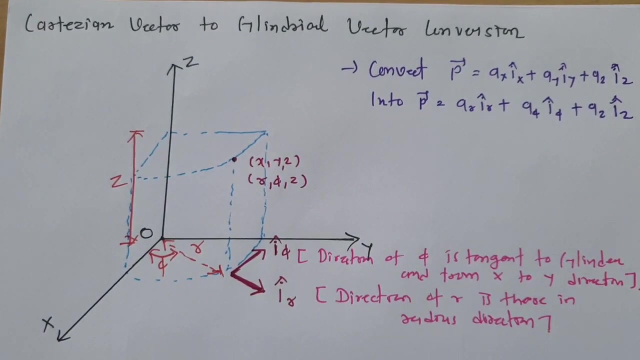 cylinder, So we can say direction of: I PHI, that is tangent to cylinder, and from X to Y. So see, that will be in this direction: I PHI, so that is So direction of PHI. I PHI, that is tangent to cylinder, and from X to Y direction. and if you observe direction, 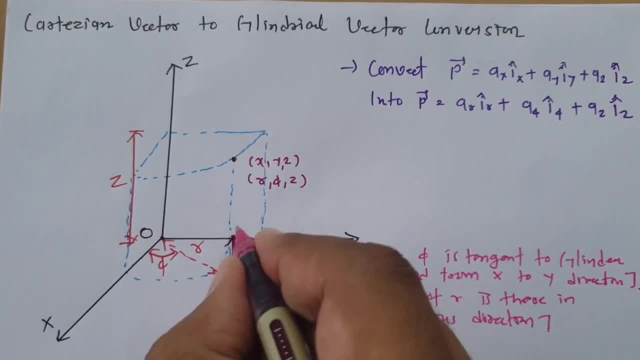 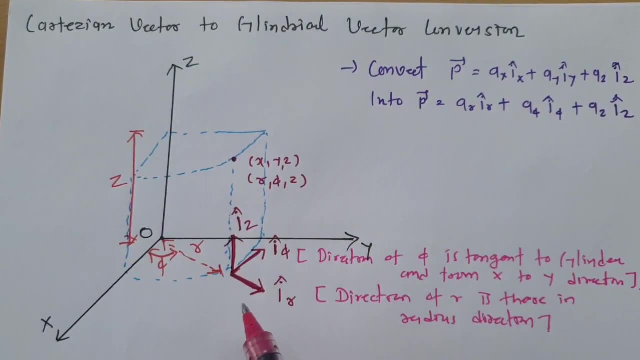 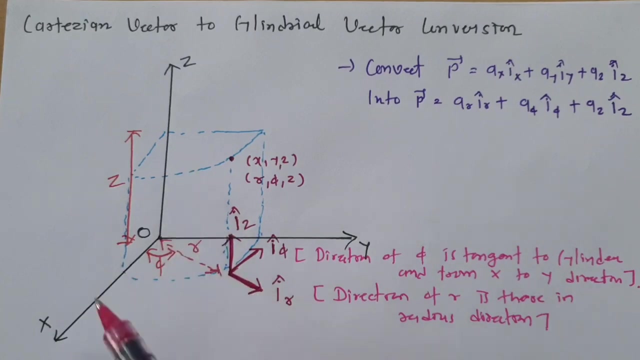 of Z, so that is same as it is there with Cartesian. so this is what IZ And if you observe all these three directions, so that is perpendicular to each other as it is there with XYZ. So direction of XYZ, that is perpendicular to each other, as well as direction of IR. 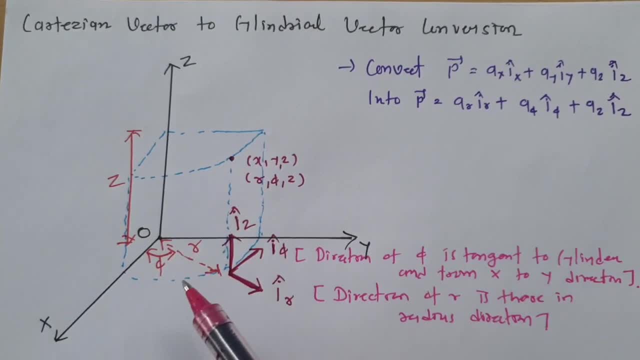 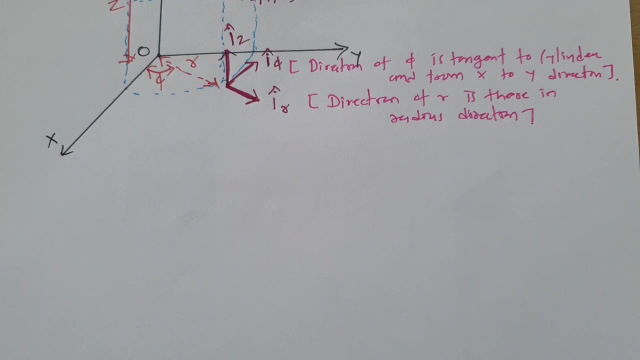 I, PHI and IZ. That is even perpendicular to each other. Now let us try to calculate AR, FI and AZ component from AX, AY and AZ components. So for a calculation of AR component, all we need to do is you just need to follow this. 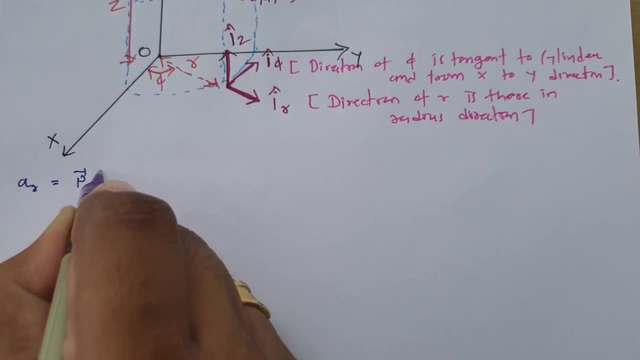 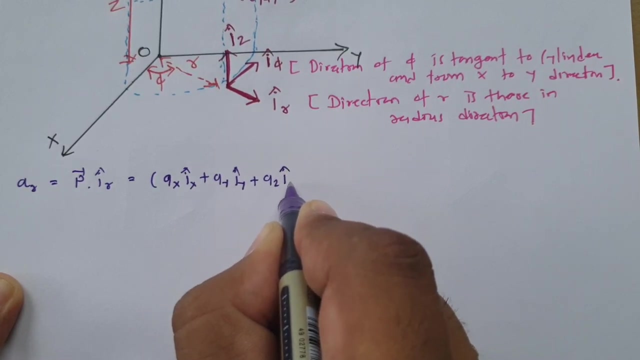 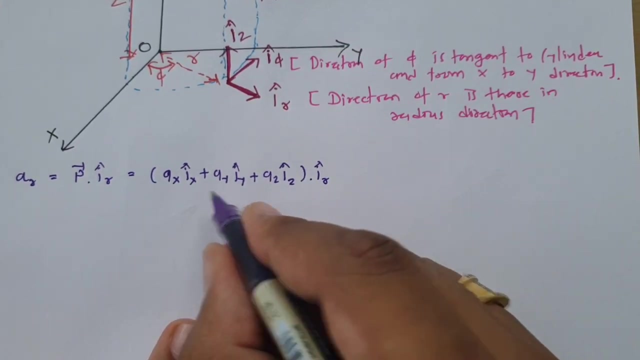 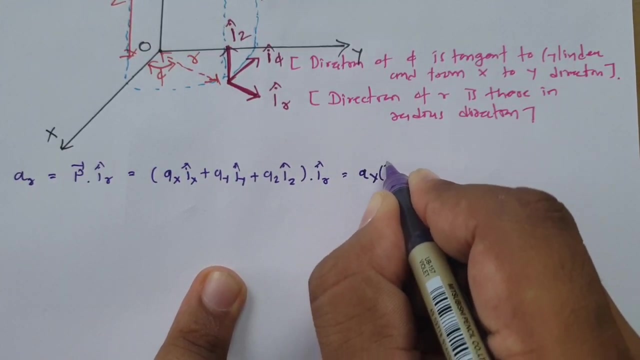 process AR. that is vector P dot vector IR. Now, what is vector P? Vector P is AX dot vector IR. Now, what is vector P? Vector P is AX, IX plus AY, IY plus AZ, IZ dot IR. Now here: if you do this dot multiplication then you will be finding this is AX into IX. 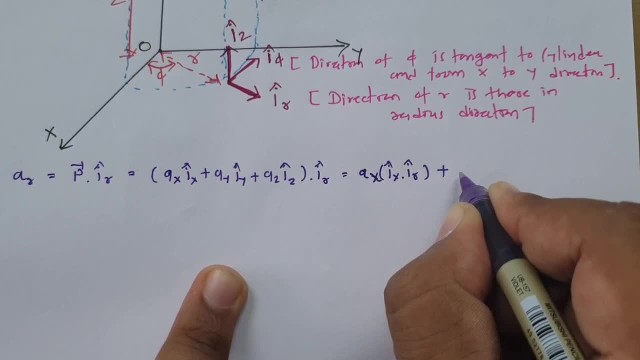 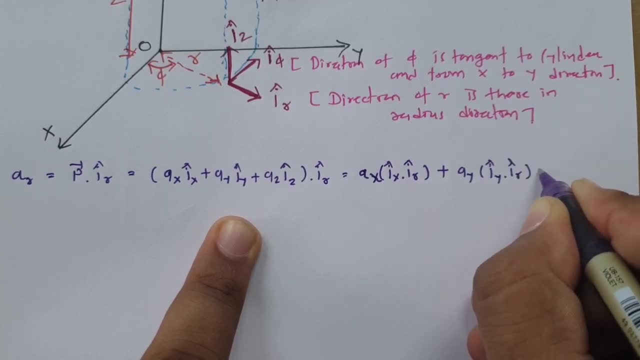 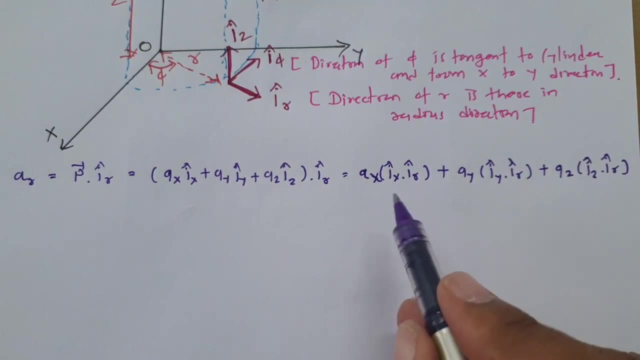 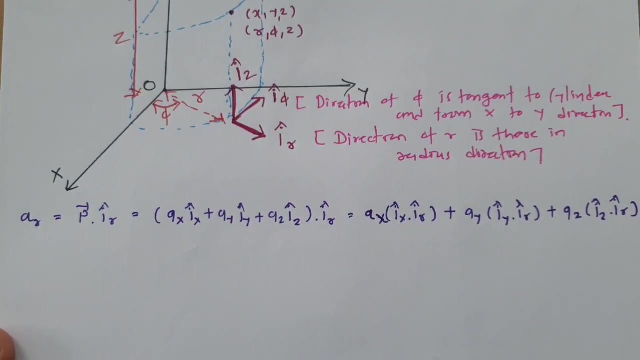 Now, what is vector P? Vector P is AX dot vector IR plus AX into IZ dot IR. Now we need to identify what is this dot for, IX dot IR. Now you see, if you observe the direction of IX, so that is there in this direction IR. 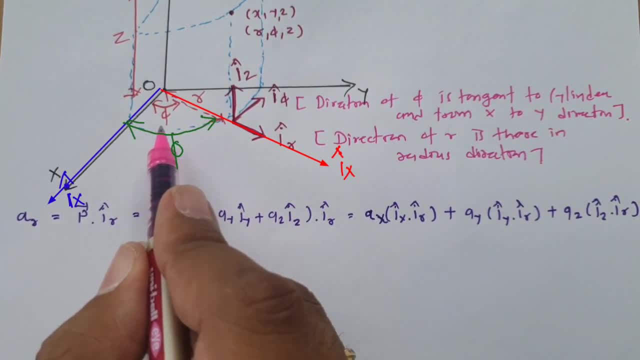 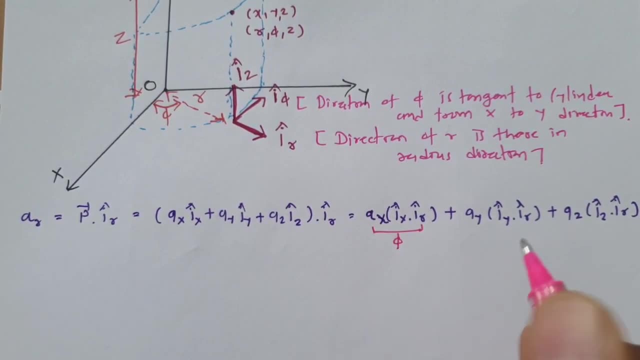 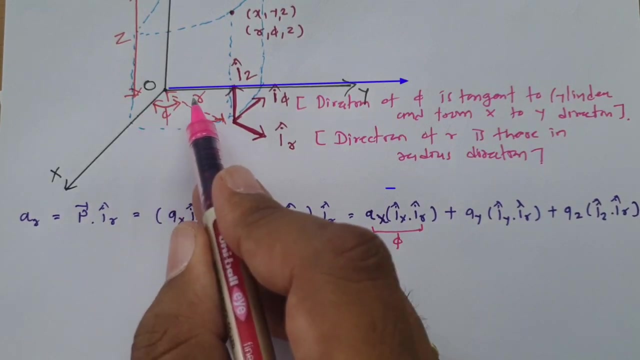 that is there in this direction, and angle in betweenanging between IX and IR, that is PHI. So let me mention over here angle in between ix and ir, that is phi. Now angle in between iy and ir. So if you observe angle in between ir, that is this, and iy, so that is 90 minus phi. 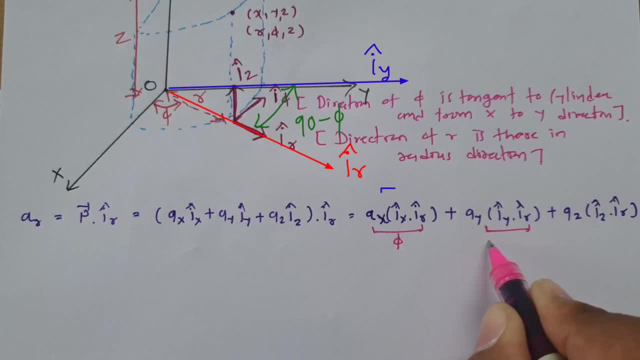 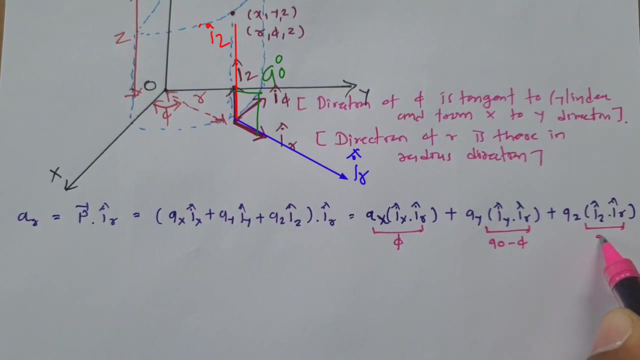 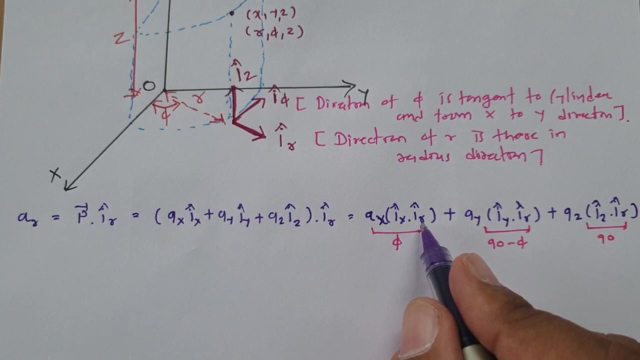 So angle in between ir and iy, that is 90 minus phi. And if you observe angle in between iz and ir, So iz is there in this direction and ir is there in this direction. So this angle is 90 degree Right. So now for a calculation of this, see ir, dot, ix, dot, ir, that is cos phi. 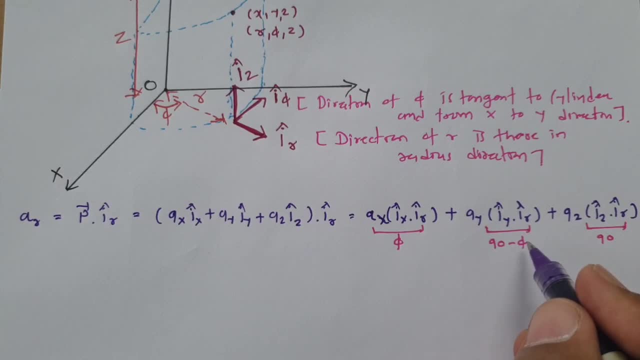 iy dot ir. so that is cos 90 minus phi. So we can say: that is sin phi and cos 90 that is 0.. So we can write this: ar, that is ax Cos phi plus ay sin phi and this cos 90 is 0. 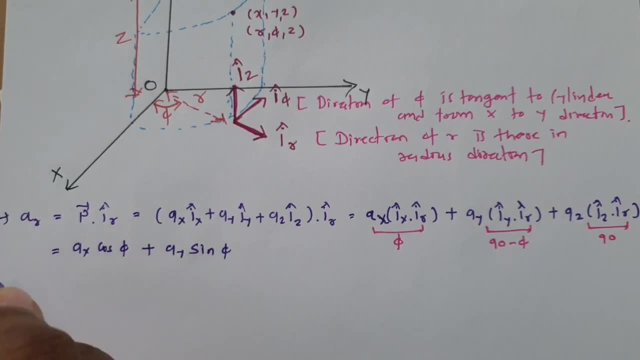 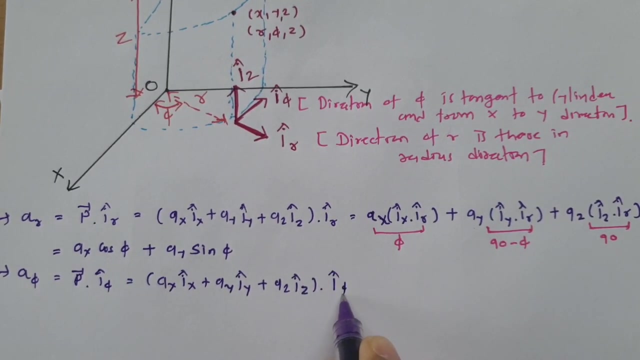 So this is what ar Now. similarly, we will calculate a phi. Now, a phi that is vector p, dot i phi. So vector p that we know ax ix plus ay iy Plus az ix Plus az dot i phi. So that is. 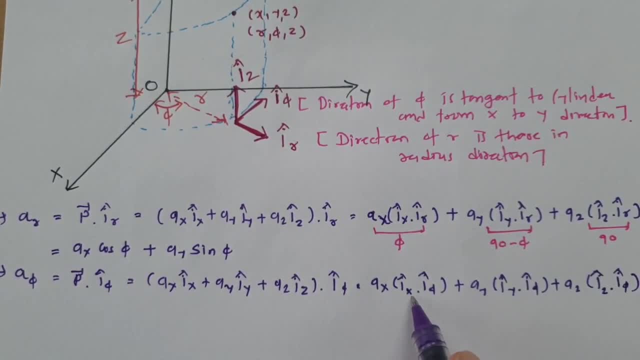 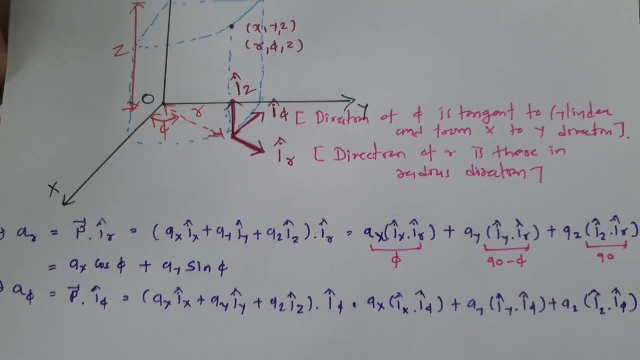 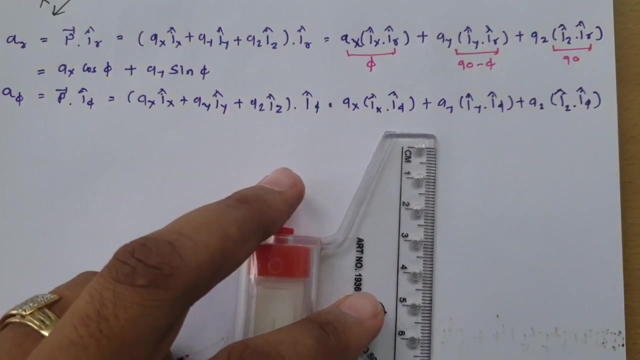 Right Now, we need to identify angle in between ix and i phi Right Now. for that we need to have top view over here. So let me draw top view first of all, So it will be giving you idea, Like how to calculate this. 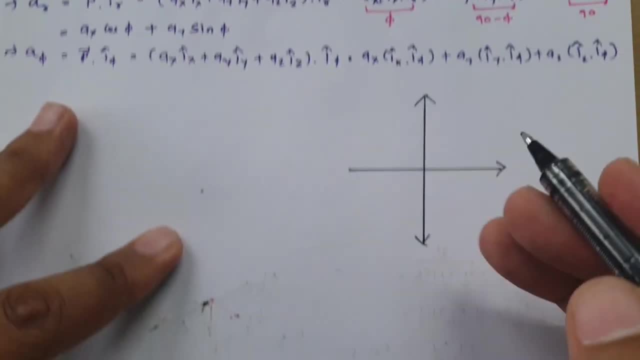 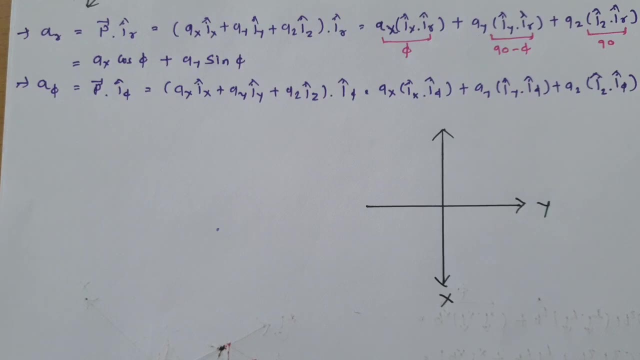 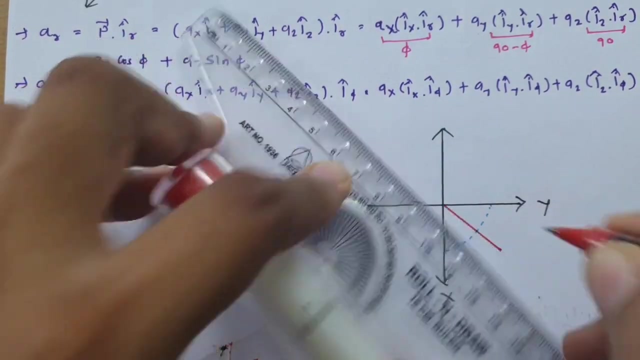 So, So, based on see, this top view is like: this is x direction and this is y direction, right, And you can see this is a trajectory like this and in this trajectory, see, this is what the direction which is there in ir direction, Right. 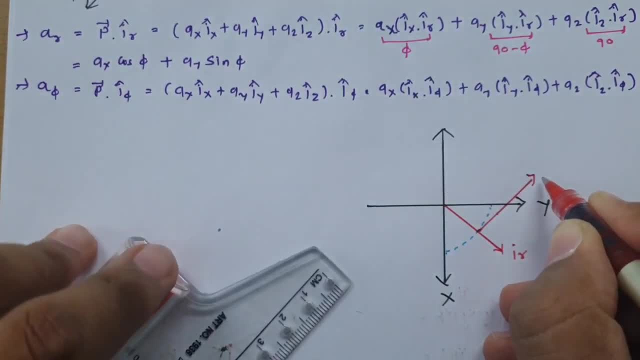 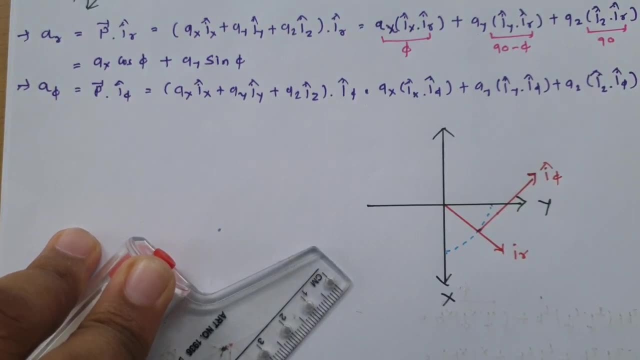 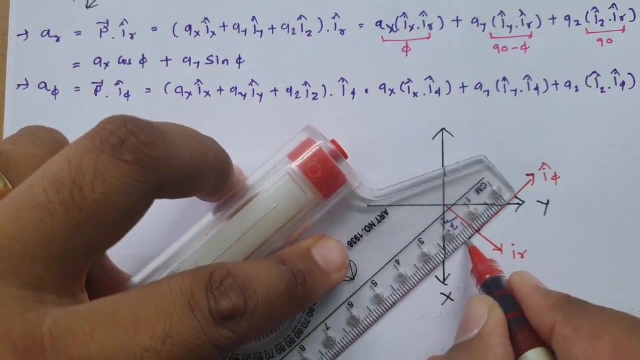 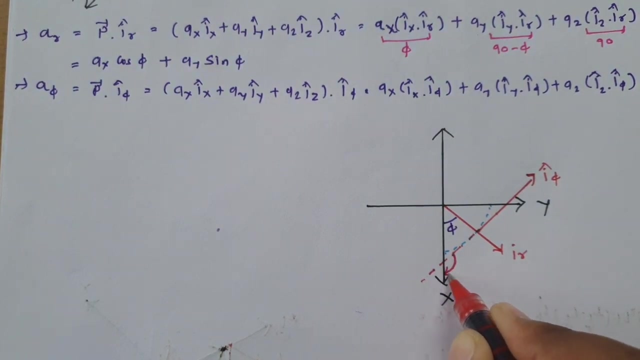 And tangent to this means this direction that is there in i phi, direction Right. And if you talk about angles, then this angle is phi. So if I take trajectory of phi in this direction, then what is this angle? So see for this angle. 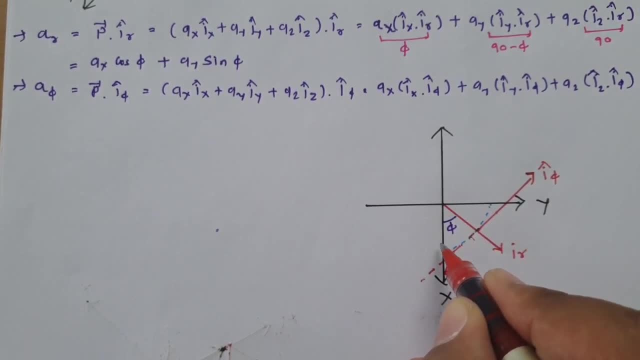 If I say this is a trajectory, If I say this is 90 degree, right, So this angle has to be 90 minus phi. So let me mention it over here. This angle, That is 90 minus phi Now, this total angle is 180.. 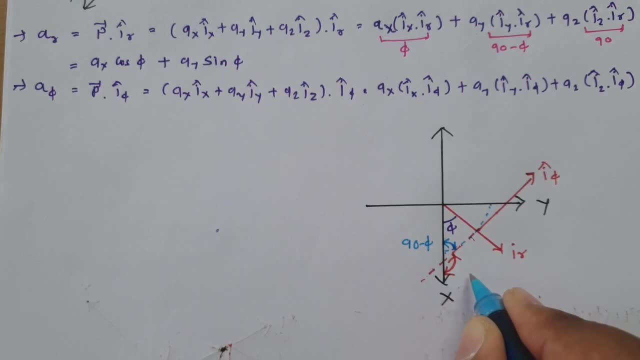 This total angle is 180.. So how much this? So this angle, That has to be 180 minus 90 minus phi, And if you calculate this, It will be 180 minus 90.. So that is 90.. Minus minus plus phi. 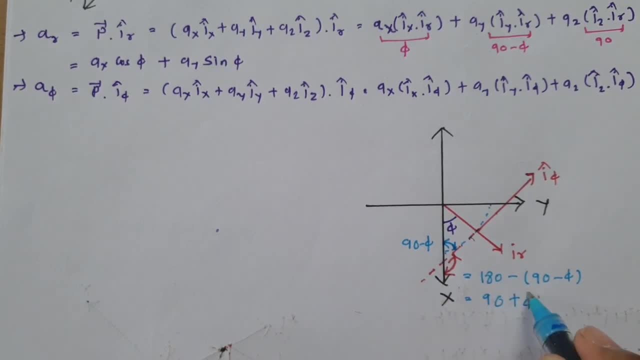 So angle in between phi and ix, That is 90 plus phi. Right. So angle in between ix and i phi, That is 90 plus phi. So let me mention it over here: This is 90 plus phi. Now, this is what iy. 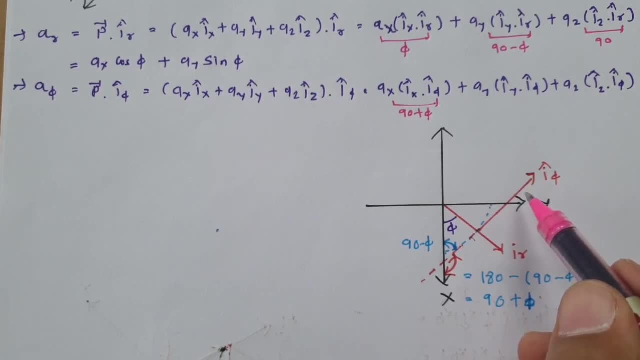 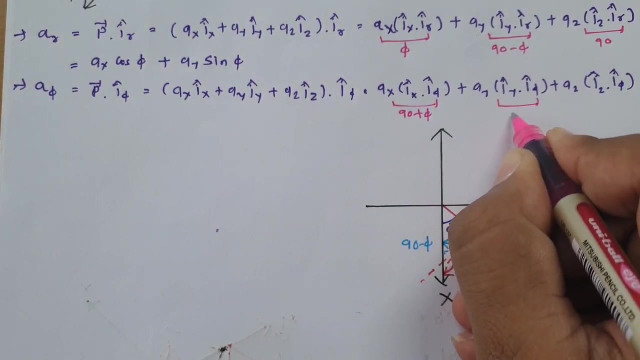 And this is what i phi. So angle In between iy and You can see this angle is phi. So this angle is exterior angle And that is even phi. So angle in between i phi And iy, That is even phi. 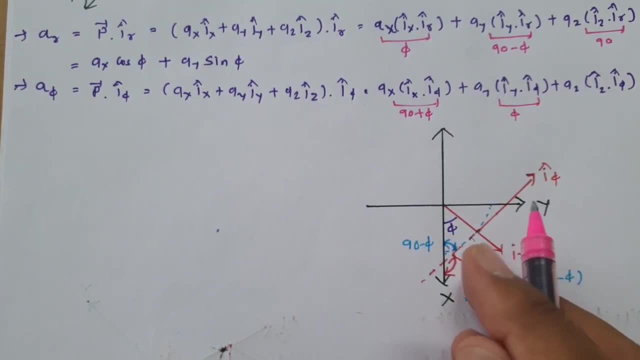 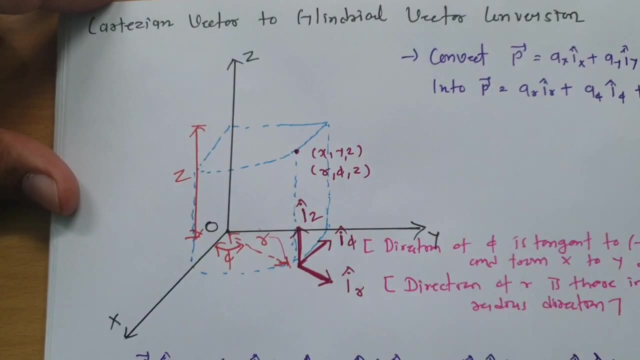 So you can say: this angle is phi And angle in between iz and phi. Iz, that is perpendicular, You can see, And i phi, that is like this. So angle in between iz and i phi, That is 90 degree. So I am writing it. This angle is: 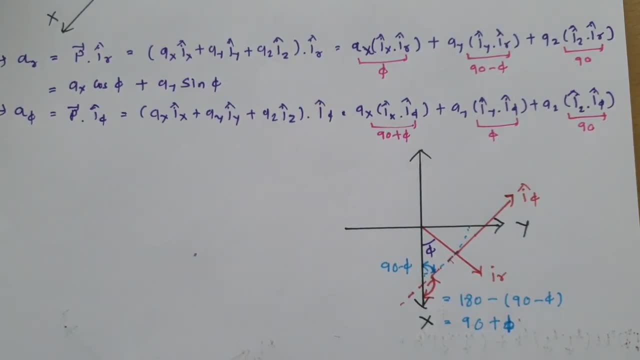 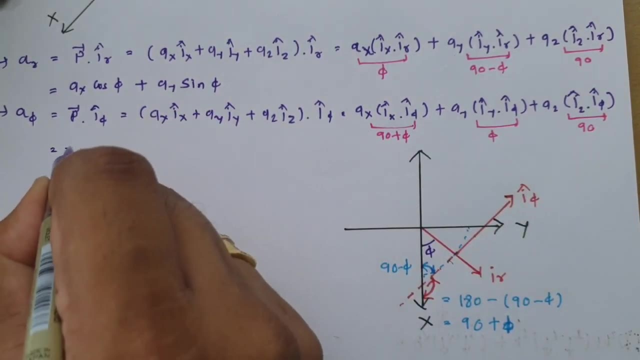 90 degree. So Now we can say: This will be Ax cos 90 plus phi, So that is minus sin phi. So we can say: this is minus ax sin phi. Iy dot i phi, That is cos phi. 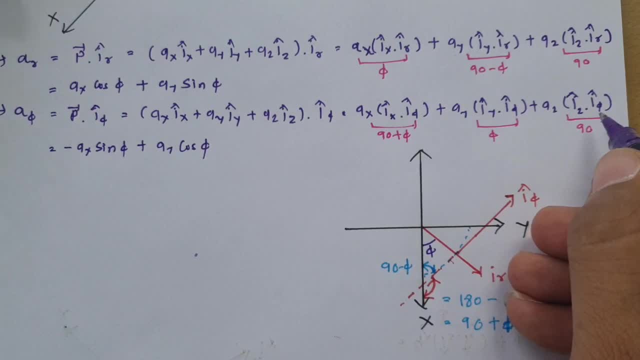 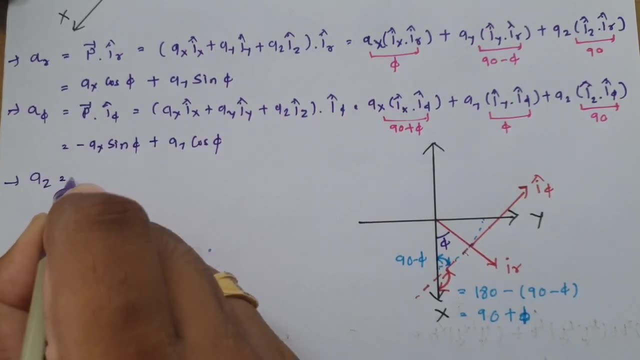 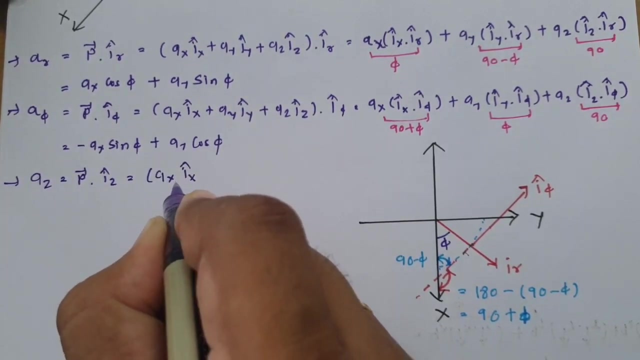 So we can say: plus ay Cos phi, And this is cos 90 zero, So we don't need to write it. And when you calculate Az, P, dot iz, And that is Ax ix, Ax ix Plus ay iy. 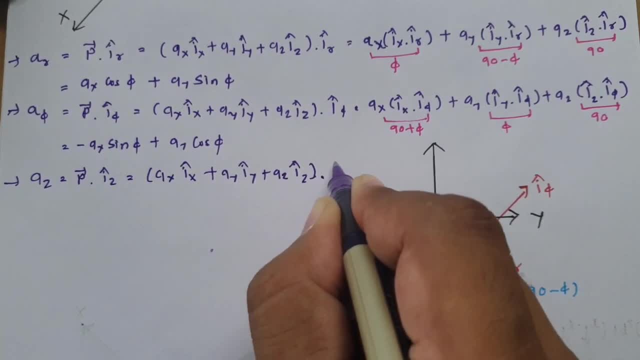 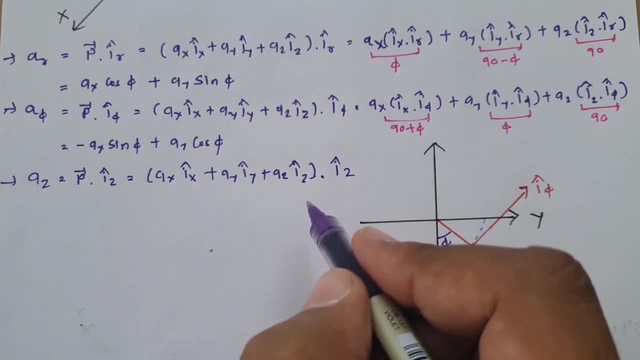 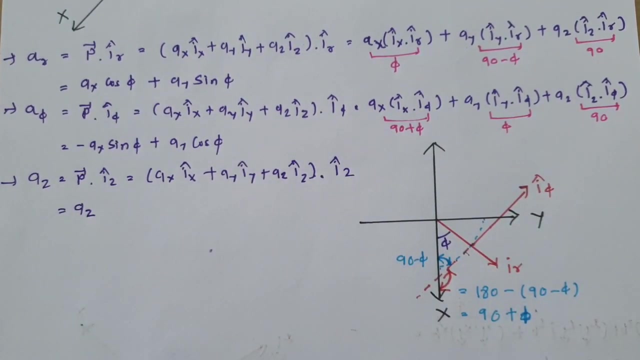 Plus az iz Dot Iz. Now here you can see: Ax ix dot iz, that is zero, And iy dot iz, that is even zero. So iz dot iz, that is one. So we can say Az is equal to az only. 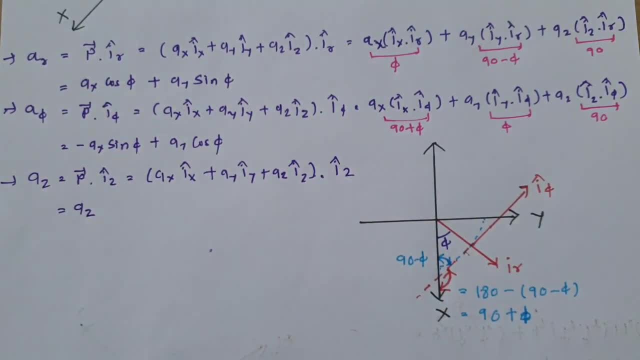 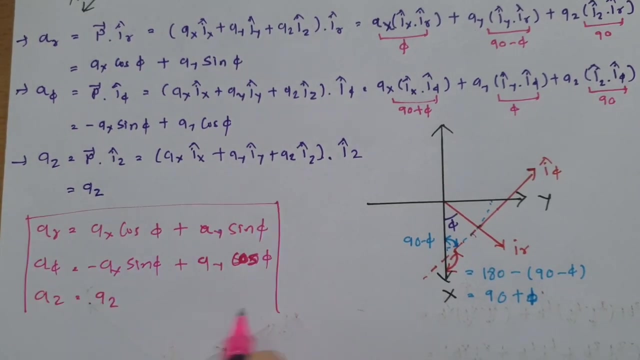 Right. So we have this Ar a, phi and az As per vector calculation, And See, this is what we need to remember, even For a solution of example. Now let us solve one example, So that will gives you clear idea. 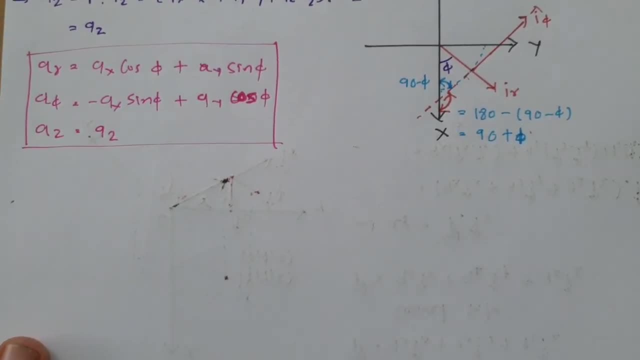 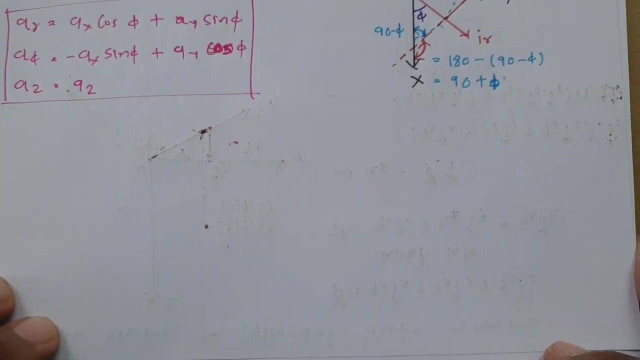 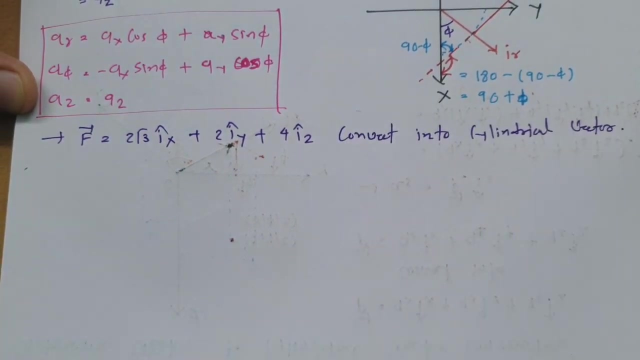 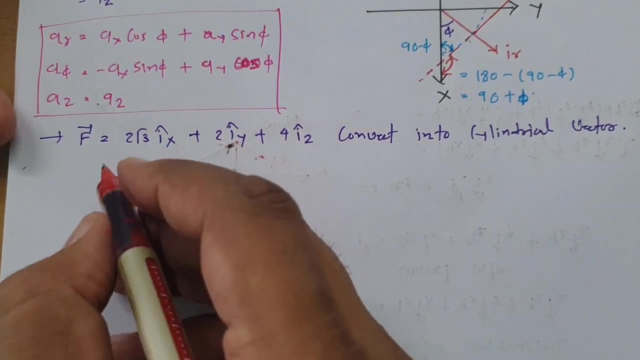 So, for example, I am just giving you One vector And Then we will solve that into Cartesian Vector. So we have been given with vector f. So here one can see, We are delivered to convert This vector into cylindrical vector. 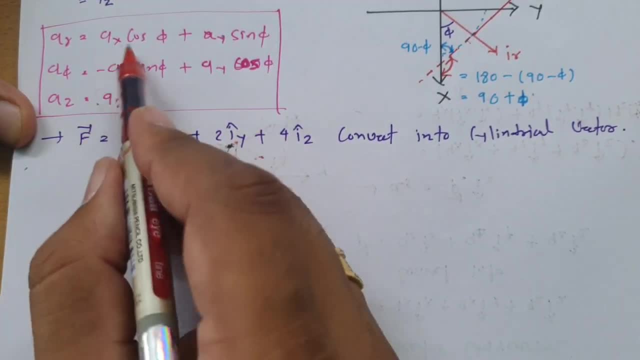 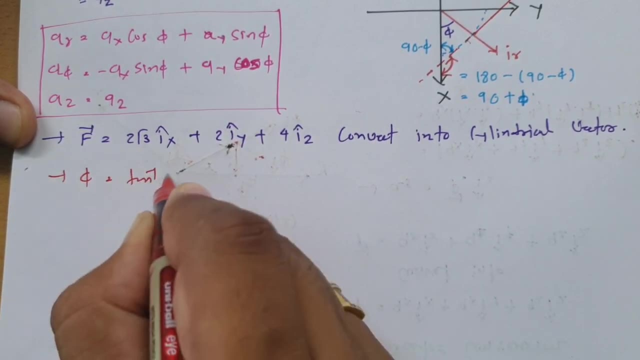 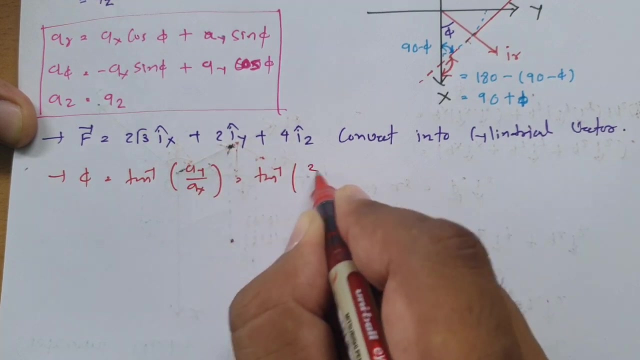 So first we need to calculate See. for this conversion We need angle phi Right. So, as we know, Phi is what? 10 inverse Ax. So 10 inverse Ay is 2.. Divided by Ax, that is 2 root 3.. 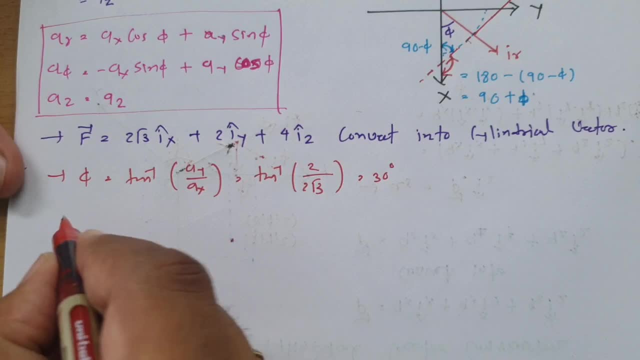 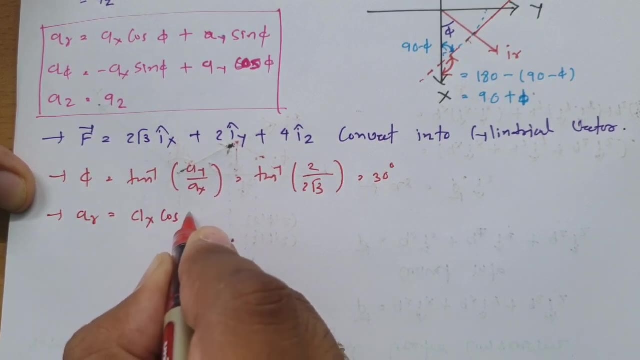 So 1 by root 3. That is 10 inverse 1 by root 3. That is 30 degree. So now we have angle phi And now we can calculate ar component. So ar component is Ax, cos, phi Plus ay.